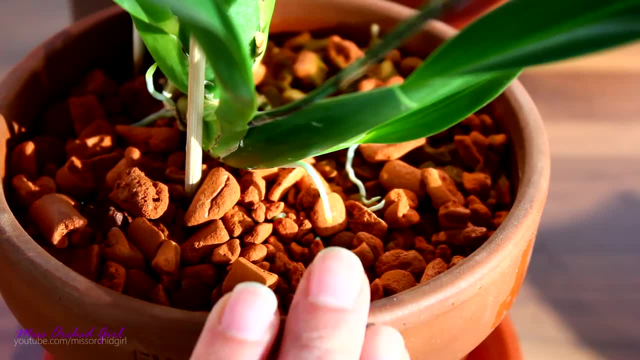 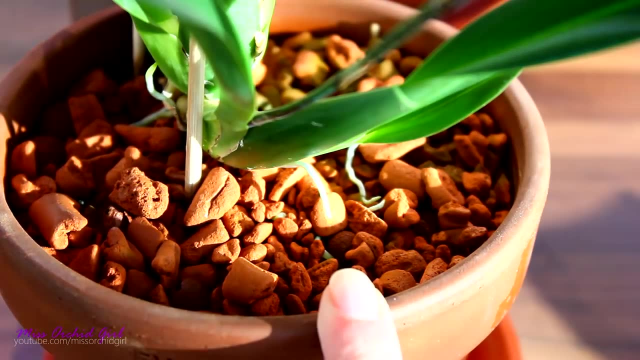 as well, but in the case of epiphytic orchids we'll add a third one and that is photosynthesis. So the best thing to do is to take each function separately, elaborate and draw some conclusions. So the first function, absorption of moisture and nutrients, pretty much like any other plant. 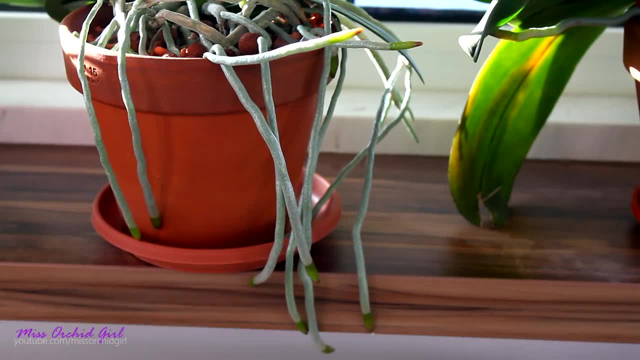 the roots on plants have two main functions. The first one is absorption of water and nutrients. the roots of an orchid are responsible with absorption of water, keeping the orchid hydrated in its entirety. They're very well specialized in doing this, as well as roots are the main organ. 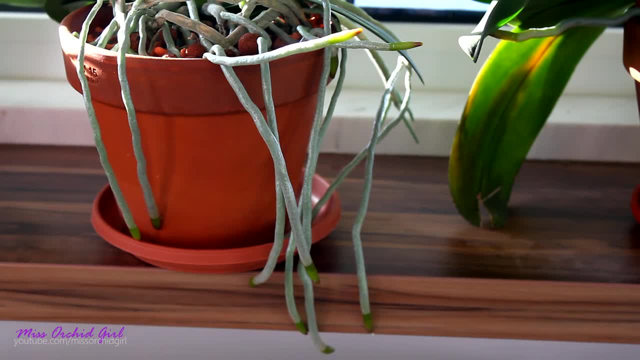 of an orchid, which are responsible with the absorption of nutrients. However, there is something special with orchid roots in comparison to other plants, and it is quite striking. On the vast majority of orchids the roots are considerably thick in comparison to other plants. 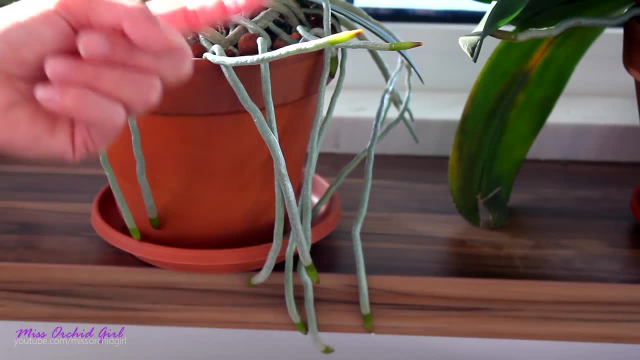 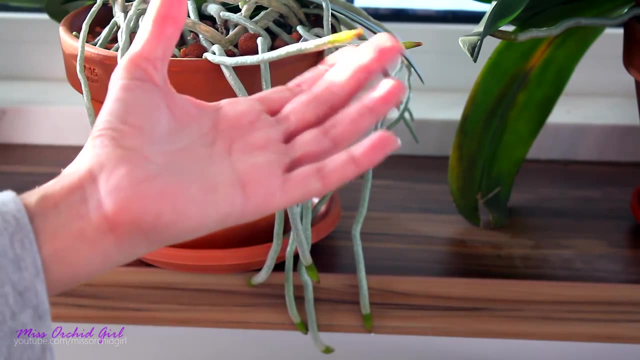 Now what's happening is that the orchid root is actually enveloped into a velumen. We call a velumen this outer coating, this fleshy formation that we can easily see, And most of the orchids we grow have this velumen, if not all of them. 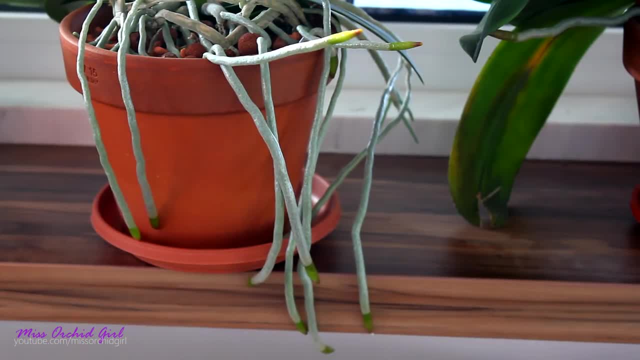 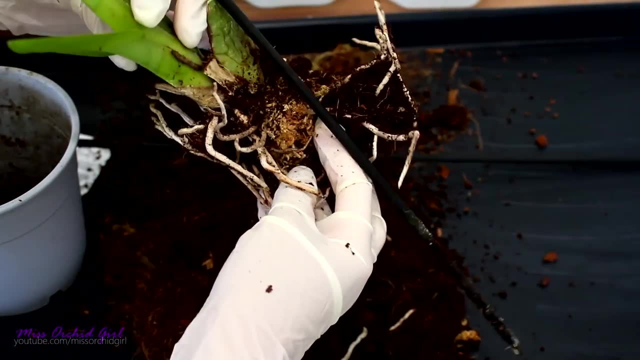 The actual root is located inside. If you've ever dealt with dead roots, you know that inside that velumen there is a very thin string That is the actual root of the orchid. The outer coating is responsible for actually absorbing the moisture and storing. 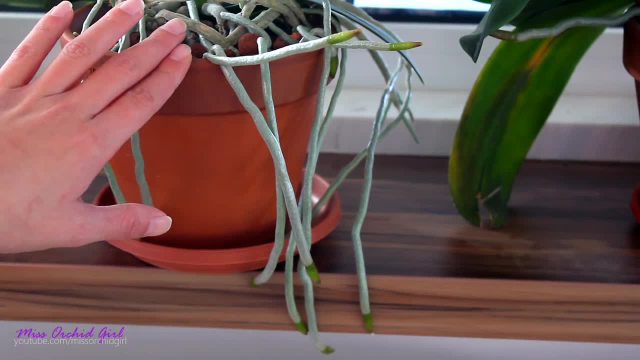 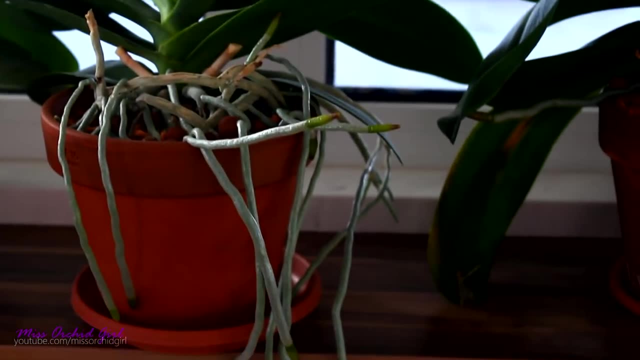 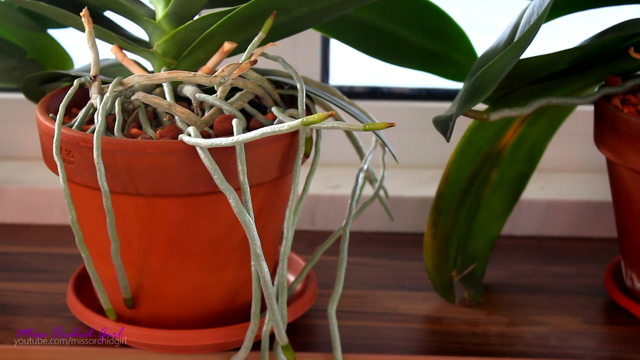 it, And the thickest roots can be observed on monopodial orchids, which means orchids that do not have pseudobulbs, like Phalaenopsis Vandas and so on. So pretty much the thickness of the roots indicates that this orchid uses roots as storage devices, not only as a means. 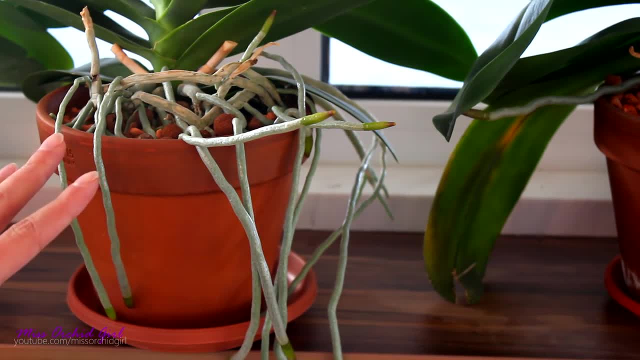 of feeding themselves. For the main part, orchids are really really adapted to withstand drought periods, And this is more obvious on epiphytic orchids, the ones that actually grow attached to trees or rocks And terrestrial display the same type of roots, very thick and fleshy. There are, however, 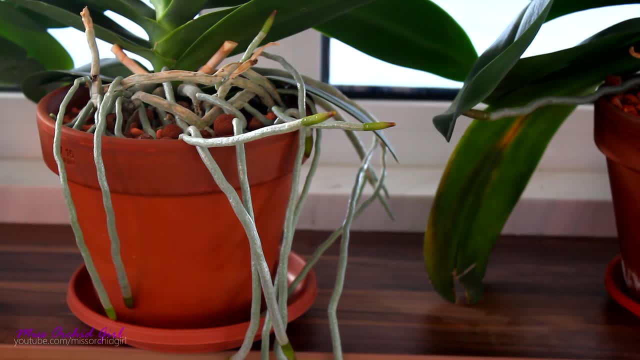 some terrestrial orchids which do not have these very thick roots. but they might have pseudobulbs or other organs And this is just an adaptation to the way they grow and their environment. But this is not a topic about pseudobulbs and all of that We are discussing. 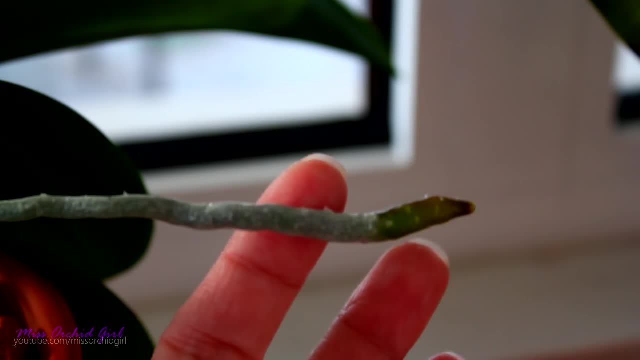 about roots. As with many other types of plants, the orchid roots are also responsible with the absorption of nutrients that are dissolved in water. Orchid roots can only absorb nutrients in a liquid form, So if you're thinking you can put some powder fertilizer on a root and 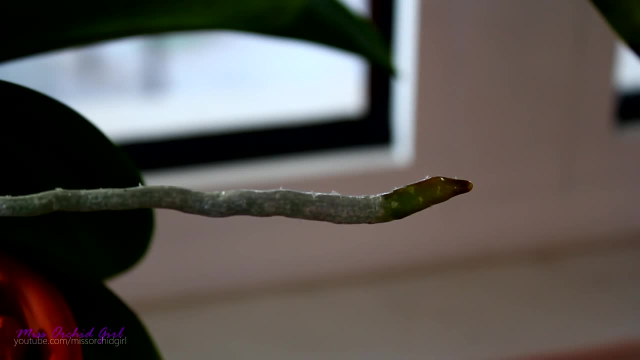 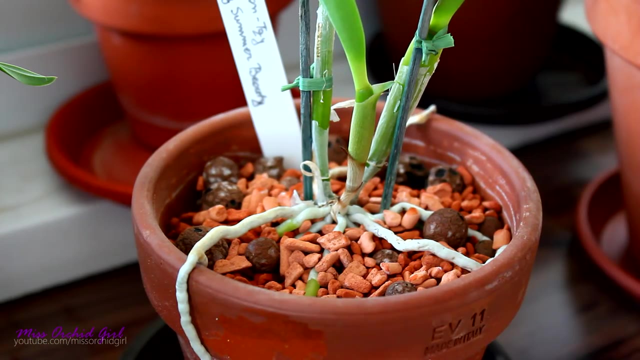 then just wait it out. it's not going to work like that. You need the fertilizer to be diluted in water for development to absorb it. Okay, the second function of an orchid root is to stabilize the orchid. When it comes to terrestrial orchids, roots pretty much behave in the same way that other terrestrial. 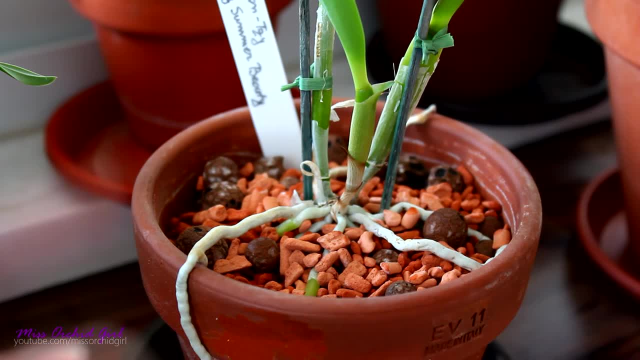 plants behave. When it comes to epiphytic orchids, though, things get quite interesting, And if you have an orchid or two, you already know that they can be used as a source of nutrients and nutrients, And they can also be used as a source of nutrients for plants. 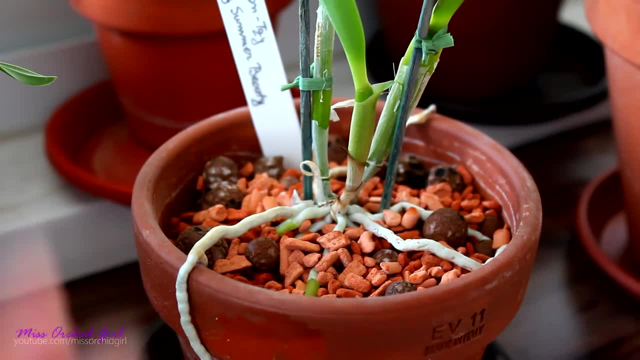 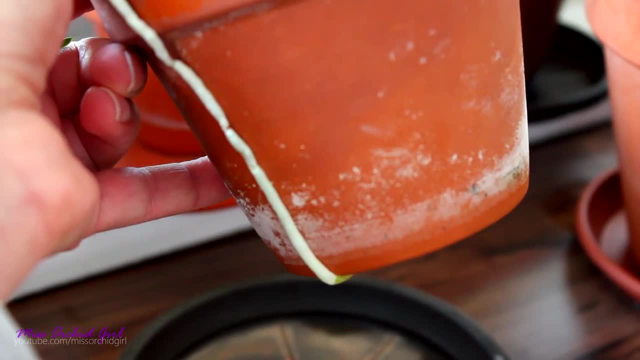 And you can use them to grow plants and plants. And if you have an orchid or two, you already know that the orchids tend to produce roots in all sorts of directions And when they reach a surface that they can cling to, they will definitely stick to that surface as strong. 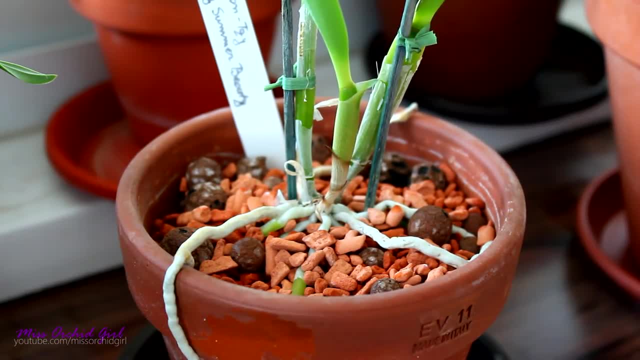 as possible. Now, this is very common with epiphytic orchids In nature. they would grow on trees or rocks or branches in any case, and not in soil, So the roots having the ability to properly attach to these surfaces is essential for the well-being of the orchid. 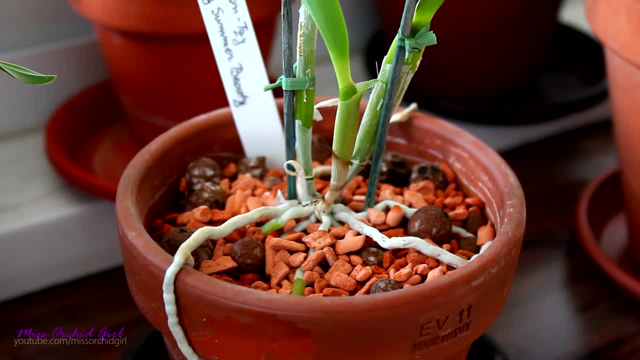 And it's not a feature of the root or a secondary function, Since location is a condition of survival for orchids, roots must be very, very capable of attaching strongly to surfaces, And not only do they need to attach very well to surfaces. 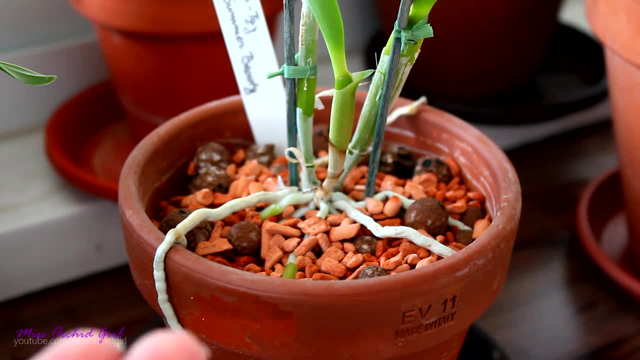 they need to know where to go in order to stabilize the orchid. So, unlike terrestrial orchids or other terrestrial plants, they tend to grow in whatever direction you can imagine: They will go downwards, they'll go to the side and they will also go up. Now, 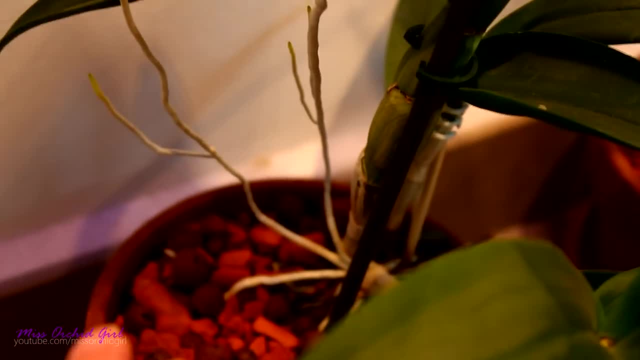 in the orchid hobby. we refer to the orchid as the root of the orchid And the root of the orchid is the root of the orchid. So we refer to these roots that actually don't grow into the pot as aerial roots. But the truth is all orchid roots are aerial or 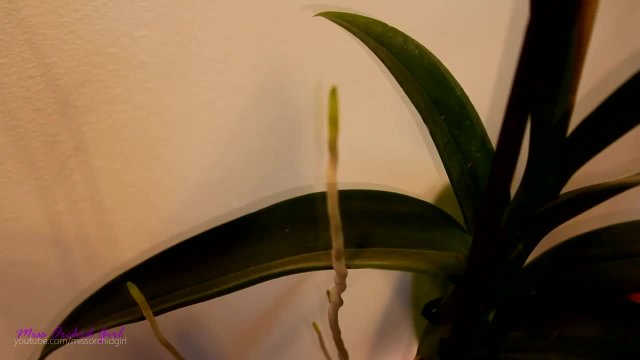 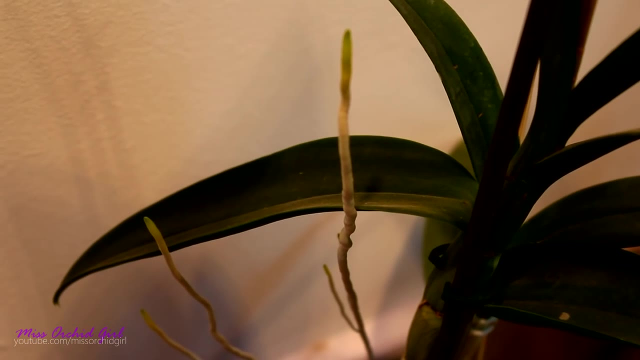 at least they have the capability to grow in air- And I am referring here only to epiphytic orchids, not terrestrial or semi-terrestrial. And when faced with this, many people are pretty perplexed. But there is a logic behind it. So let's imagine that this orchid is 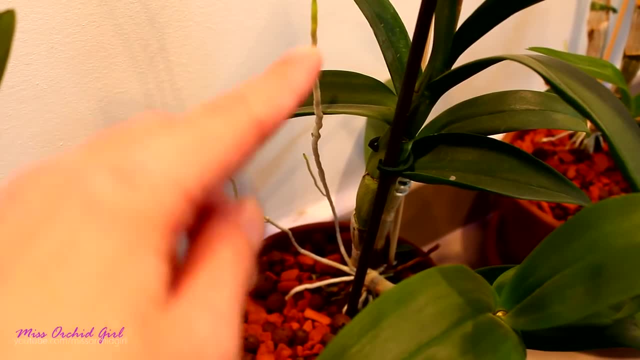 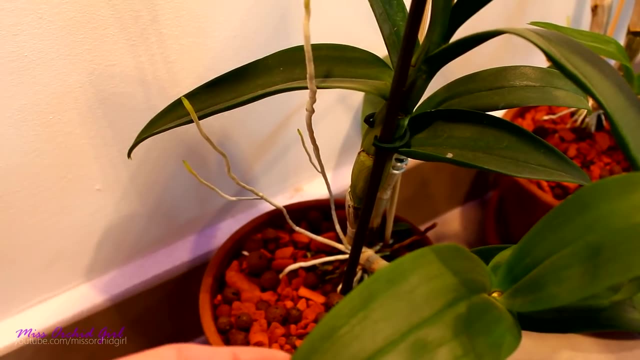 not potted, But behind it it would be a tree. The roots will try to go up the tree, but the roots will try to go down the tree to anchor the orchid from above. They will also grow sideways and also down the tree. In this way the orchid is super secured on that tree. 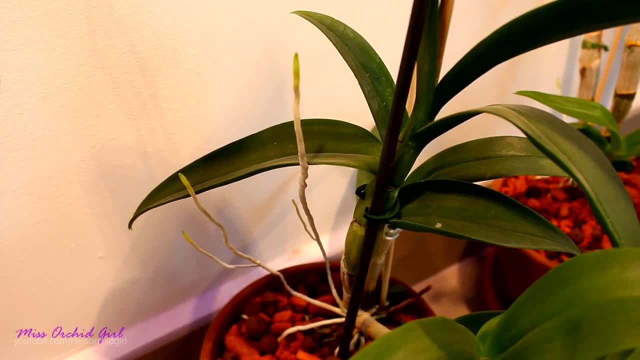 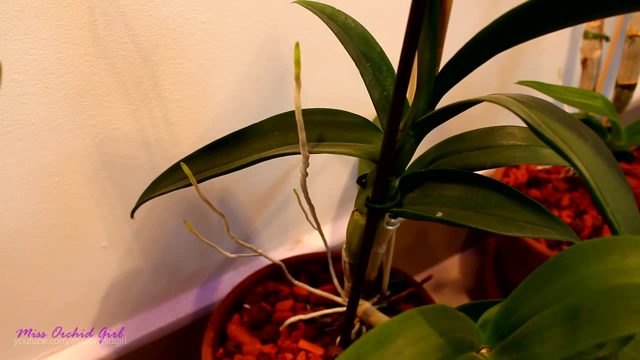 and no matter how strong the wind is, it will not fall. As I was saying, it is a condition of survival. If an orchid falls from its tree, most probably it will die. it will get eaten by an animal, it will rot, who knows. really, It is absolutely essential for the orchid. 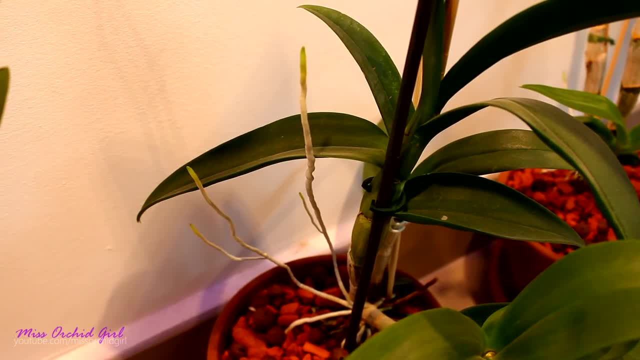 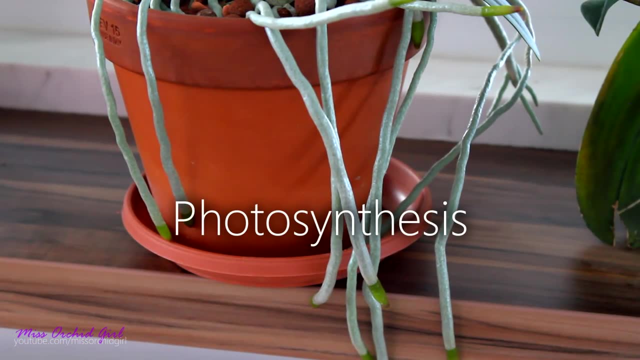 to remain in its location. Thus, anchoring is a very important job that the roots perform. And the third function is photosynthesis. This is more of a side function of the root, in the sense that the orchid already has a very specialized organ that handles photosynthesis. 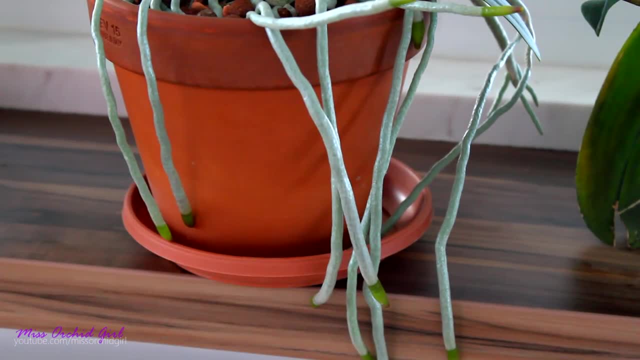 much better than the roots, and this is the leaf, But we'll discuss about this more when we talk about leaves. Roots, however, are able to photosynthesize as well. Since they grow in air, they have adapted this side feature as well. It is not essential for the 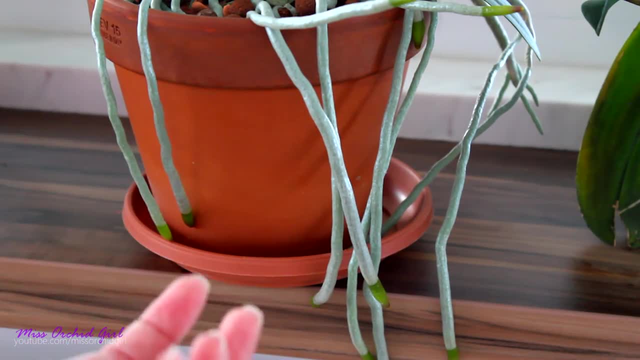 well-being of the orchid. but it is a bonus And this will be more obvious if you are in situations of crisis such as the orchid loses its leaves. The photosynthesis produced by the roots will help the orchid recover faster, But in the overall health of the orchid, 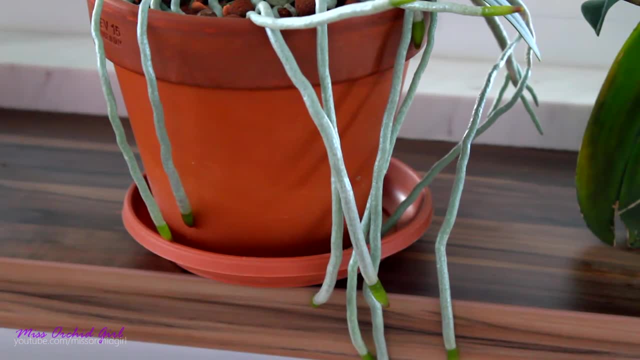 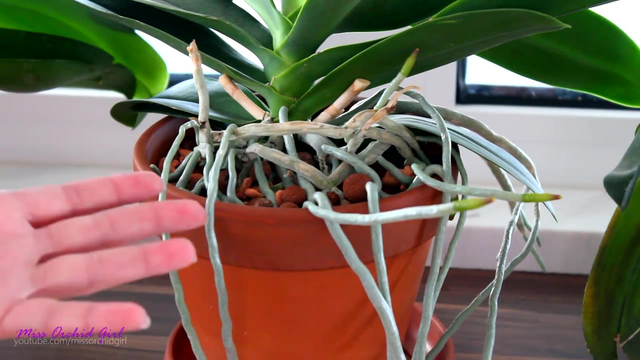 considering. we do have a healthy orchid. the big job still relies on leaves. Now this function of the roots appears more obvious when we water them. When orchid roots are dry, you can see they appear to be slightly silvery, And this is because the velumen is. 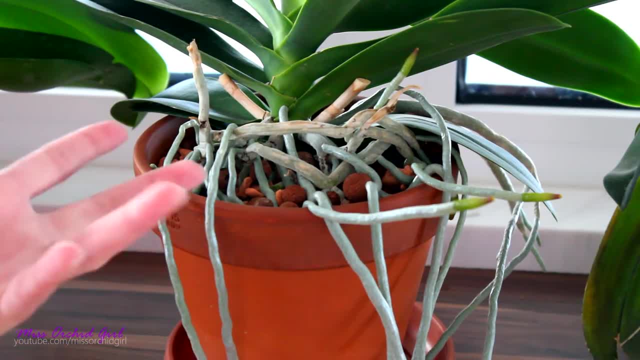 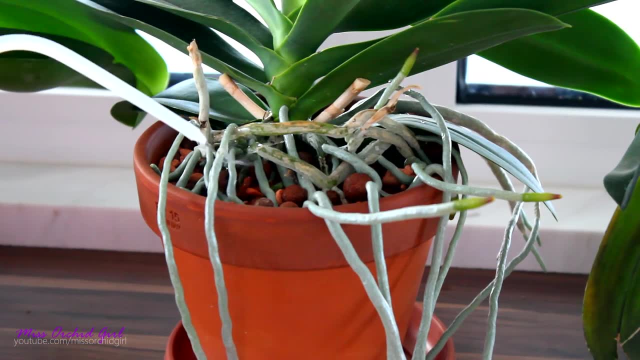 a translucent covering, but when it gets wet it becomes silvery, And I shall demonstrate. As you can see, when watered and when the velumen starts to absorb water, the roots turn green, And this is because, on the inside, the velumen is capable. 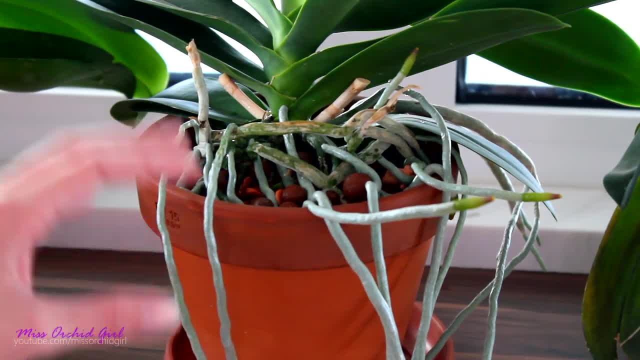 of photosynthesizing. The roots will only photosynthesize as long as they have light. If the roots grow in a dark location, such as my clay pot, which does not let light come in, they will not be green. It doesn't mean they're not functional or that they're sick. 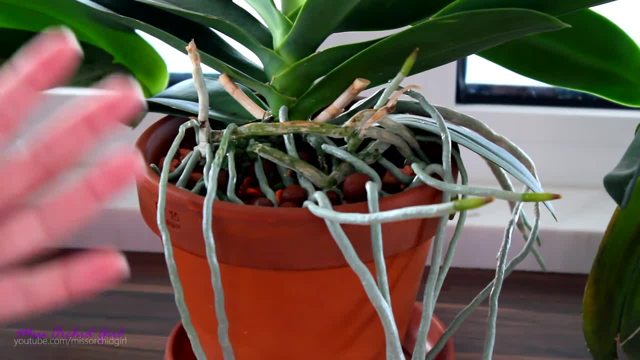 And I've talked about this in a different video. It only means they do not have light. Thus they do not photosynthesize, But, as I was saying, this is not a main, main job for them, So they can perform their other duties very well without photosynthesizing. 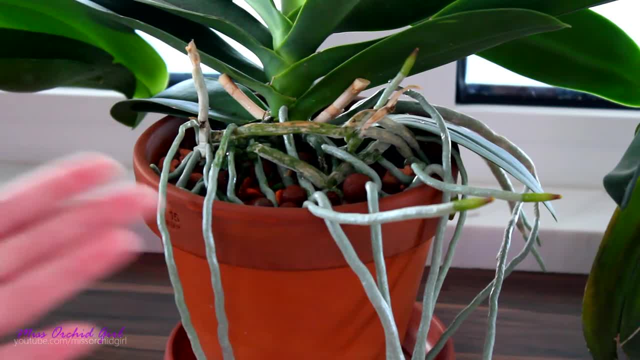 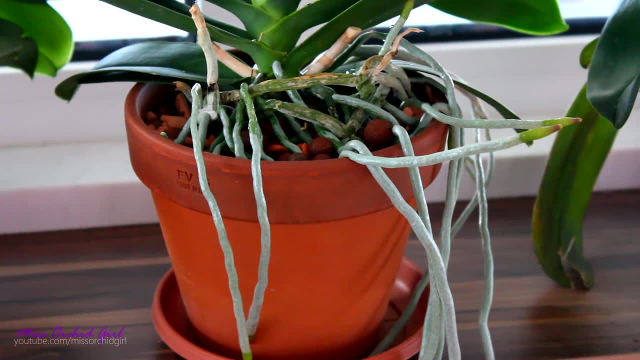 as well, But aerial roots that are exposed to light will always photosynthesize. So knowing these three functions of orchid roots can actually help us grow our orchids better and can prevent us from making quite big mistakes. One of the most common questions. 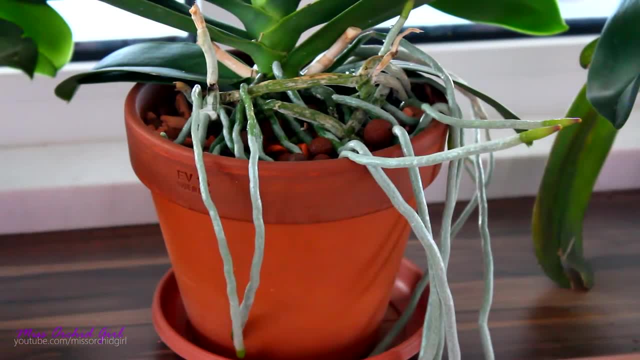 that I get is: can I cut the aerial roots of a orchid? And my answer would be no. it's not a good idea. In optimal conditions, if you cut the aerial roots, maybe nothing bad will happen. But as we all know, in the orchid hobby, things are unpredictable. So presuming something, happens with the roots that are inside the pot. like root rot, the orchid will benefit from its aerial roots. They are still capable of absorbing moisture, even though they're growing in the air, And actually they are absorbing the moisture in the air. 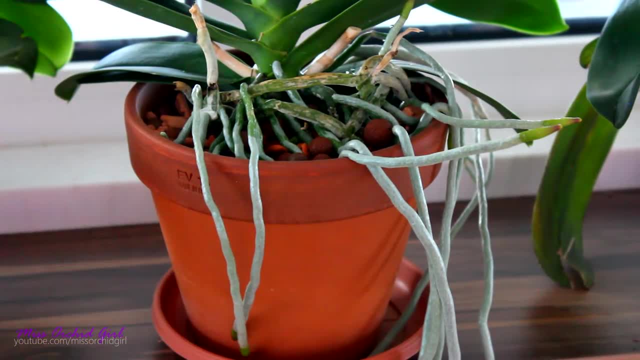 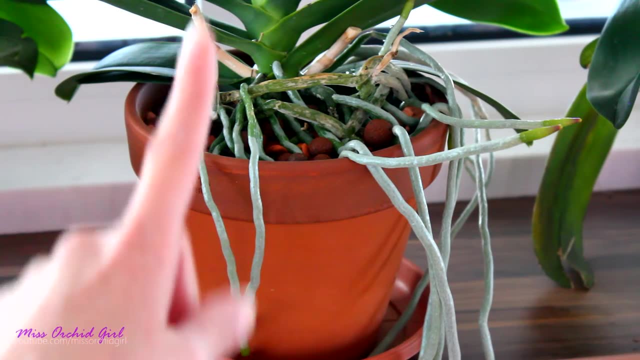 If an orchid manages to lose all of its potted roots, you can simply mist the aerial roots And in this way, the orchid will get hydration. So, if you will, the aerial roots are plan B, And you never know when you're going to need the plan B. 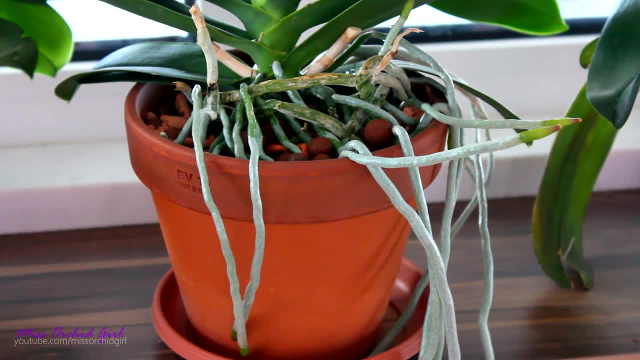 Also, let's presume that you managed to lose all of the leaves on your orchid. Maybe you kept it too much in the sun. it suffered from severe sunburn, Who knows? There are so many cases in which you can actually lose the leaves of an orchid By having aerial roots to photosynthesize. 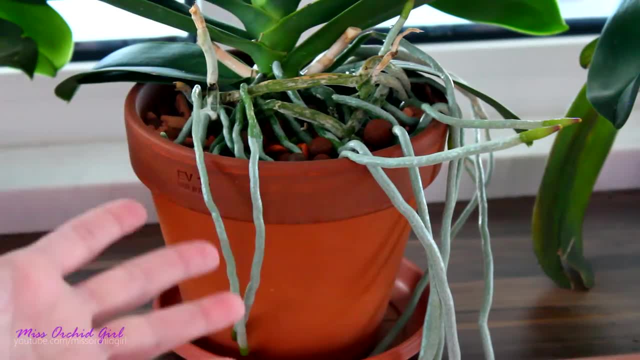 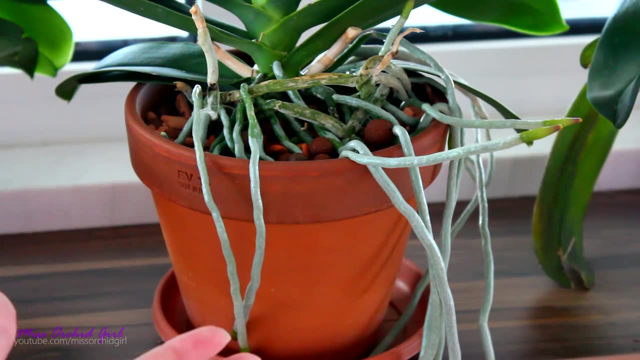 you are making sure that the orchid stays in the sun for a long period of time And it still has a future and has a help in producing more leaves, Because leaves are not free. They cost an orchid, energy, And by energy I mean the sugary sap produced after photosynthesis. 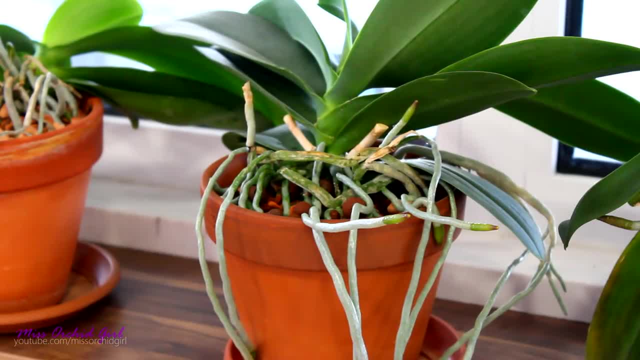 And who better to give a helping hand than the aerial roots? Now, even though the photosynthesis created by the roots is not enough to maintain an orchid healthy, some orchids actually depend on the photosynthesis produced by the roots, For example, Chylokista orchids. 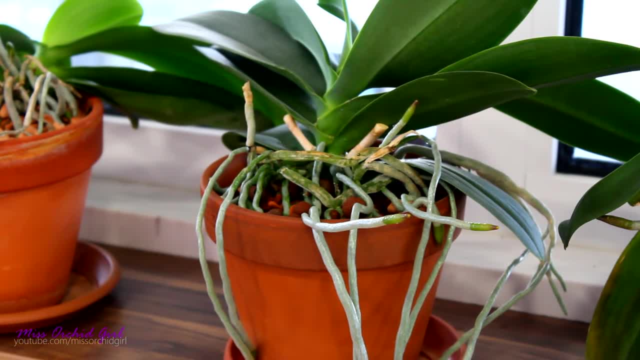 Now that species of orchid does not produce leaves. So whatever photosynthesis the roots produce is enough to maintain that orchid alive, enough to maintain new roots growing, existing roots living and even produce flowers. But the catch is that orchid does not have 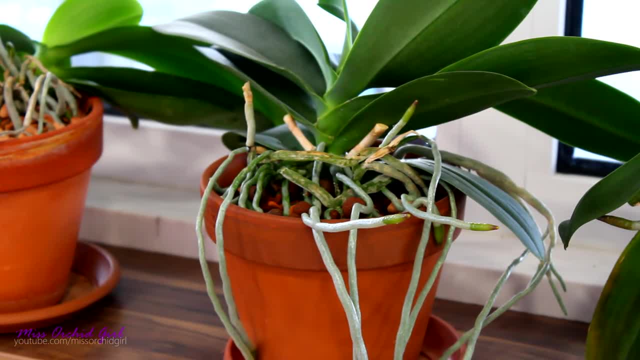 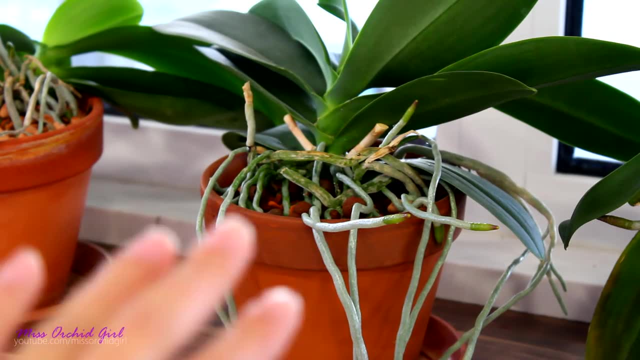 to spend energy on producing leaves, So its balance is different. If we take a Phalaenopsis or another leafed orchid, things are different. The root system alone cannot photosynthesize enough to maintain healthy leaves, And that's why photosynthesis is so important. 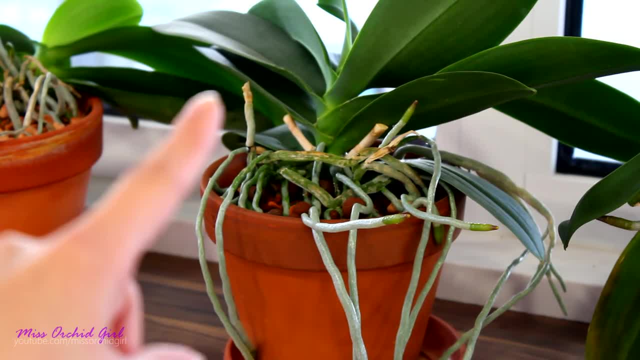 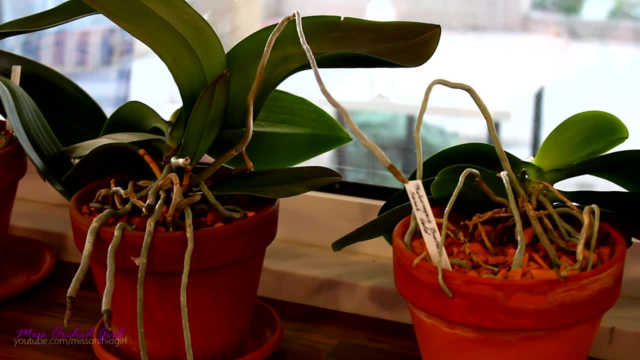 Thus, the leaves are the main organ responsible with the photosynthesis, But we'll talk more about this subject in the video regarding leaves. Now let's get back to the second function of the roots, which is anchoring. Many people have so many theories that roots actually grow towards moisture that they grow away. 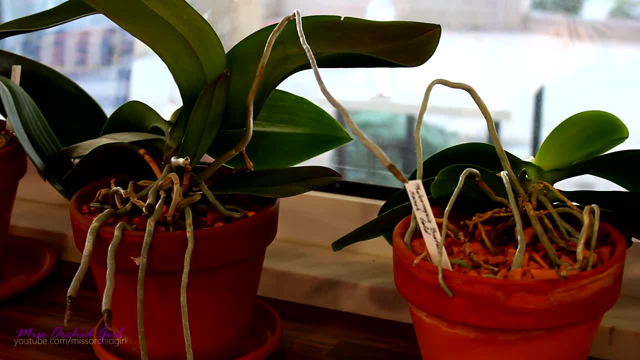 from the light, or they actually grow into the light, and so on. It has gone as far as to say that if orchids produce aerial roots, there's something wrong with the medium and you need to repot it because they grow outside. 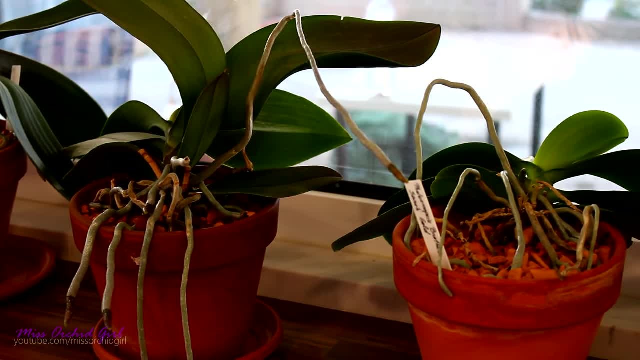 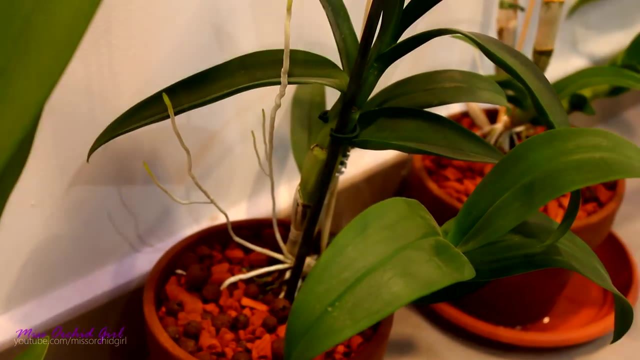 That's because they don't like the medium. And the truth is, nothing is 100% true. I'm willing to accept that roots will behave in certain ways in extreme cases, But let's take each theory and debunk it So, as we saw earlier, roots can grow in different directions, As we see in this example, the 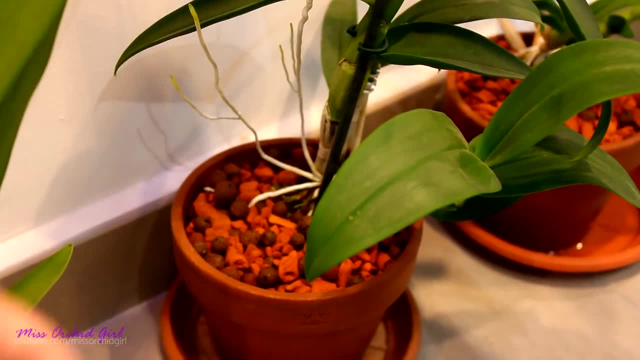 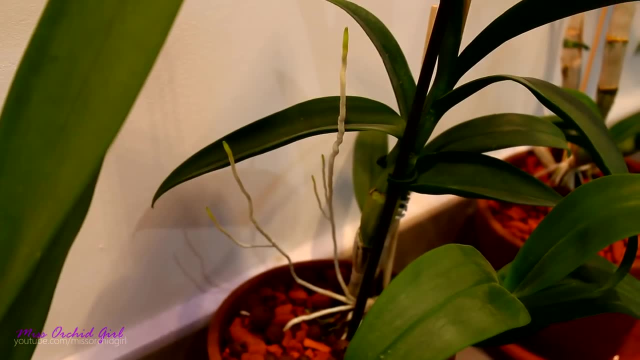 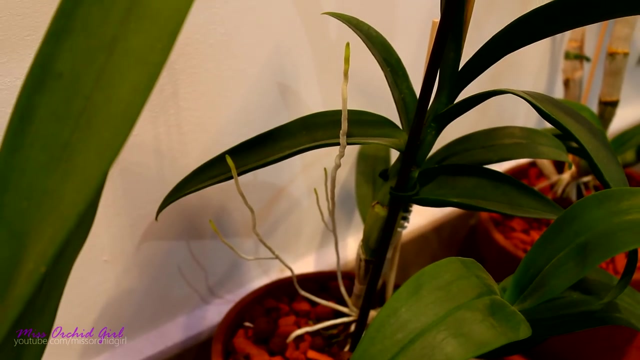 vast majority of moisture is located downwards, inside the pot. Outside there is considerably less moisture. So are these roots actually growing towards moisture? Highly, highly unlikely. We can also assume that they're growing up because they don't like the medium. But if these guys 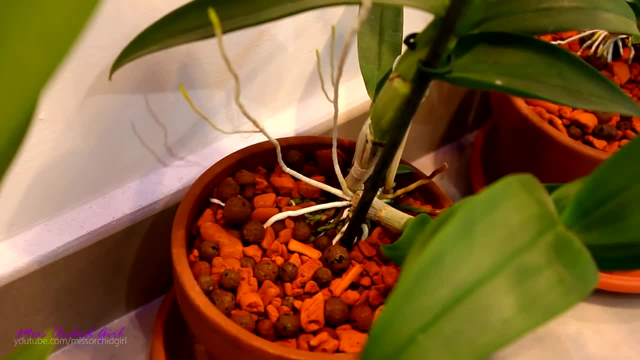 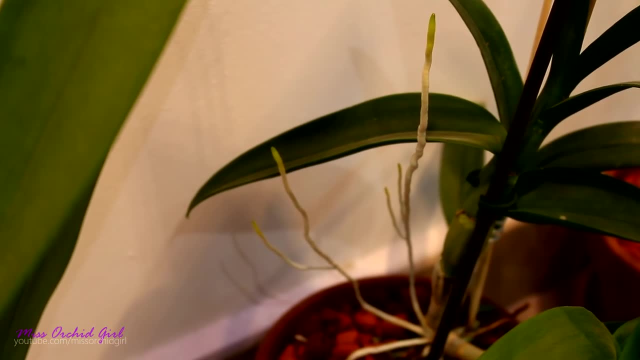 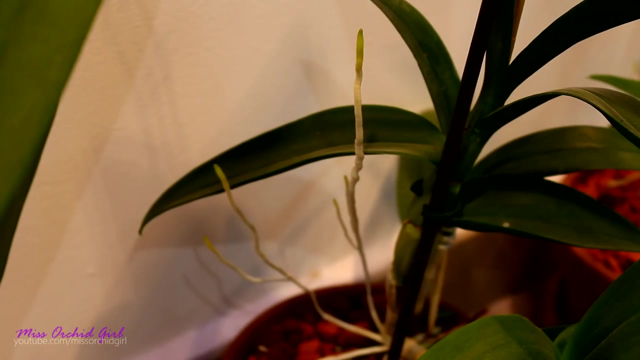 are growing into the medium, and actually most of them are growing into the medium. how come these ones didn't like medium? Are they different? Well, not necessarily More plausible is the anchoring aspect. If an orchid is anchored in all directions on a tree, chances. 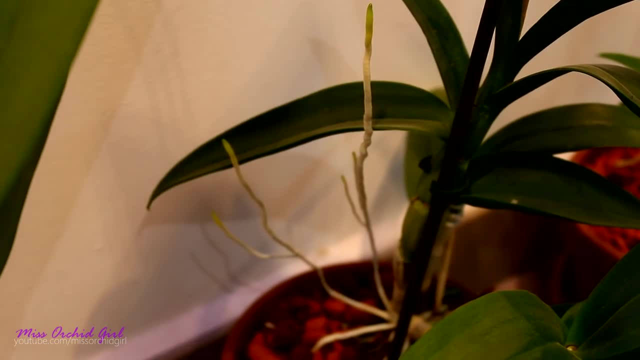 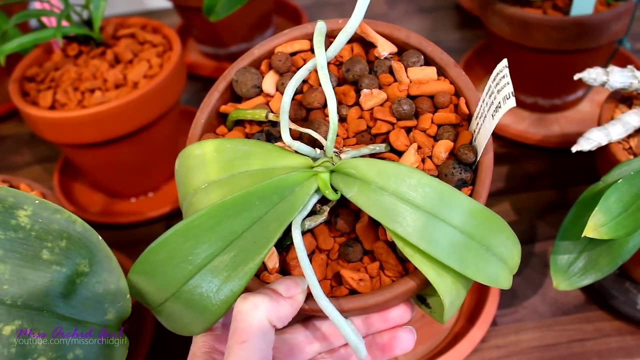 are. the orchid is anchored in all directions. Let's take a theoretical example. So let us take this orchid In nature. it would grow something like this anchored to a tree. As you can see, my roots are growing quite in different directions, Even inside. 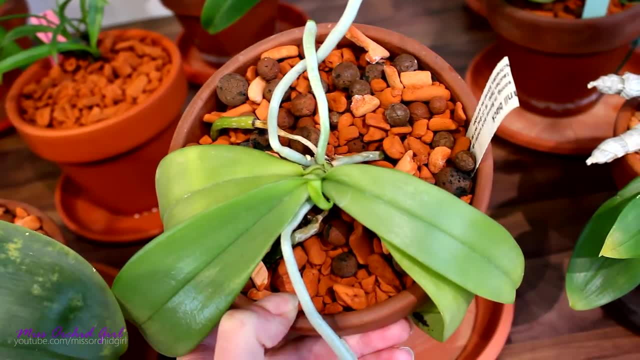 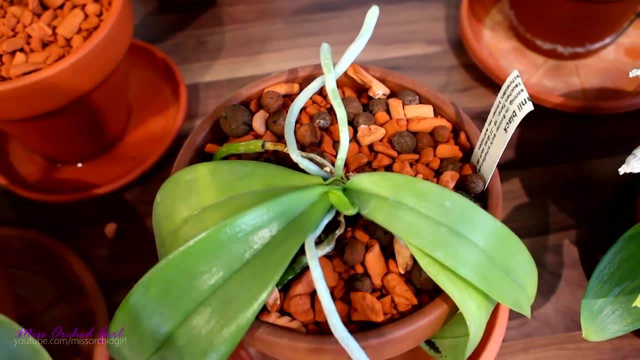 the pot outside, lower and above the orchid as well. Now if this orchid would encounter moisture on this side only theoretically, if the theory would be correct that roots grow towards moisture, every root should start to grow in that direction. 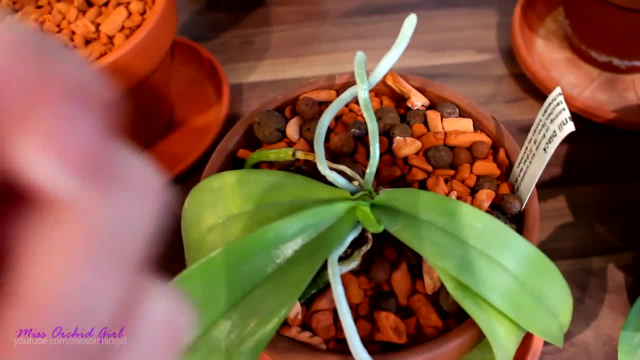 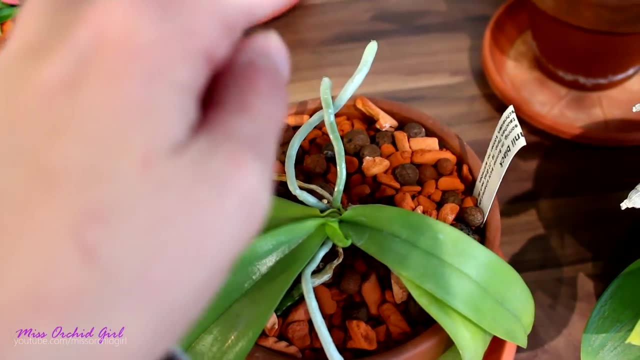 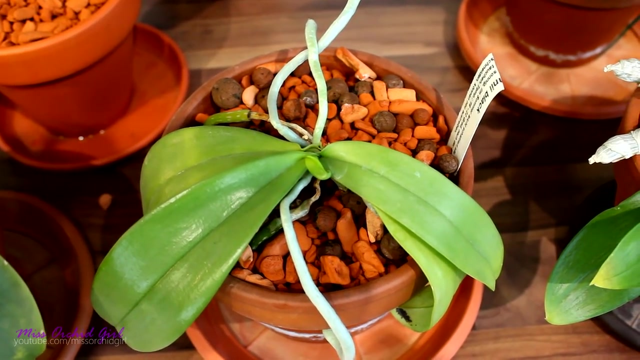 What would happen to the orchid? It will kinda start to flop in the wind, And that's not okay. When an orchid starts to flop with all of her weight, chances are the roots will snap, And the orchid really doesn't want that. So it's very counterintuitive that roots only grow towards. 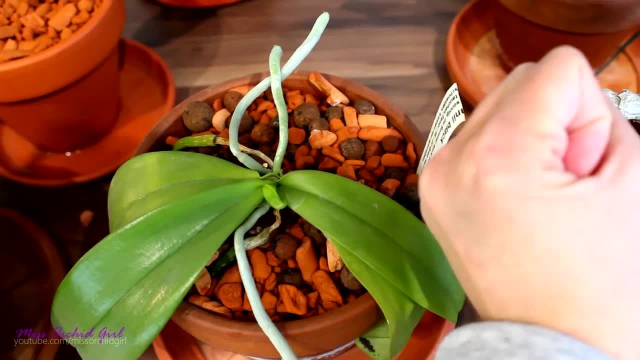 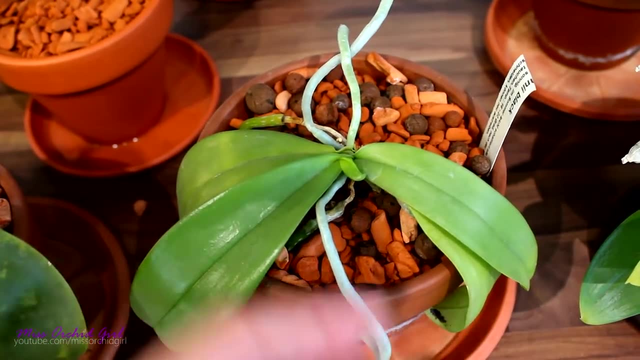 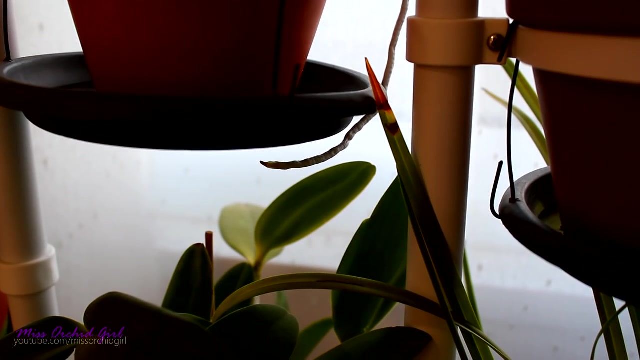 moisture, Because if the source of moisture is located here or below the orchid, there is no chance that this orchid will stay anchored on the tree if every root starts to grow towards that source of moisture. Regarding the theory that orchids grow away from the light again, it's not always the 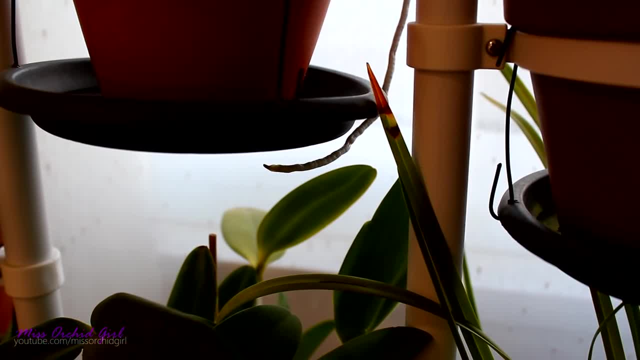 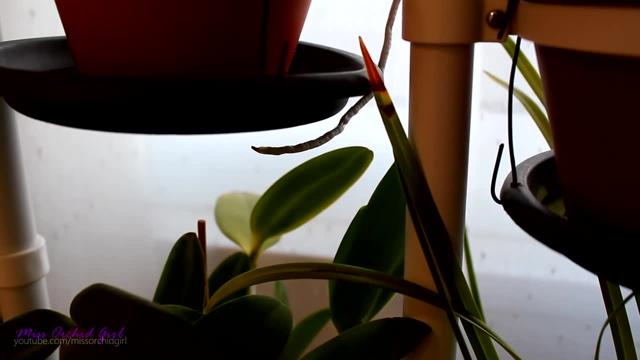 case and it's kinda counterintuitive. Since roots can photosynthesize, why would they grow away from the light? So in your collection, the more orchids you have, the more patterns of growth you will see. You can see roots growing away from the light, but you will. 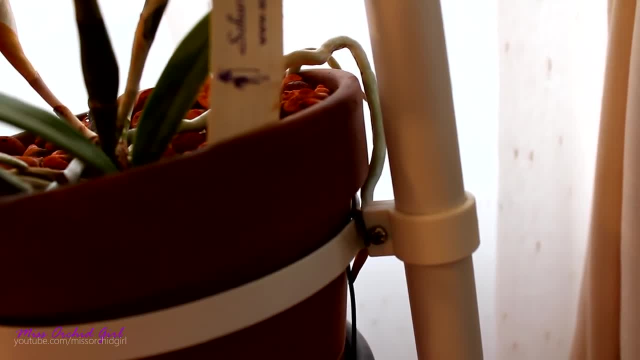 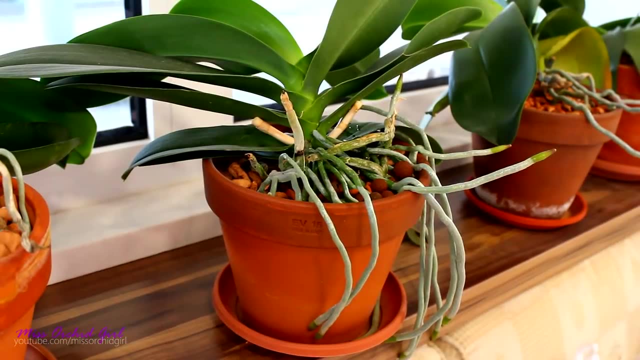 also see roots growing into the light or in the direction of the light, And the more you will observe roots, the more you will reach the conclusion that the pattern is pure. Now, as I was saying, I don't believe there is a strict rule regarding to orchids. It simply. 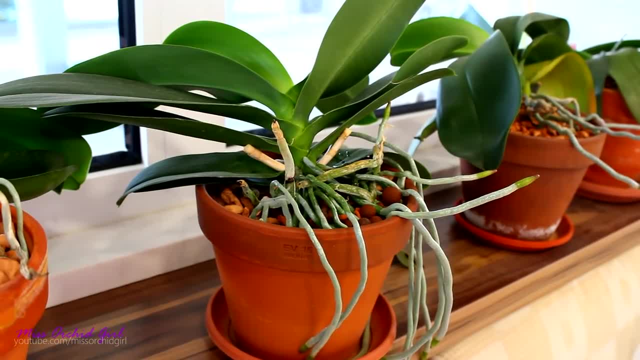 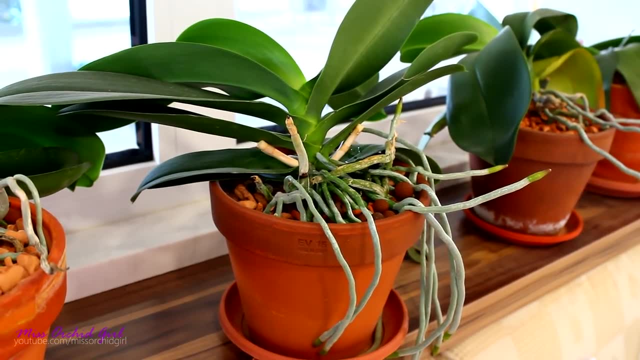 doesn't make any sense to me and it's simply counterintuitive to the well-being of an orchid in nature. However, I do tend to agree that sometimes, in extreme cases, roots tend to follow a certain pattern. So, for example, if you have inappropriate medium, I believe 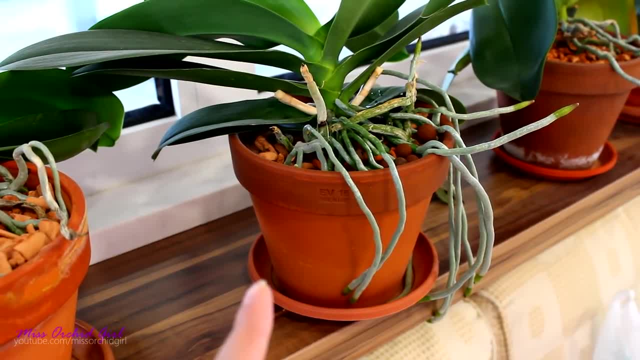 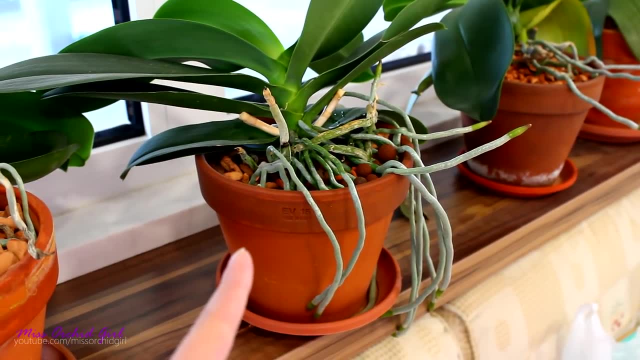 roots will tend to grow out of the pot, But in this instance you will probably notice an extreme in the sense that all of the roots will grow away from the light. So if you grow outside the pot or you will have one little root in the pot, that doesn't look too. 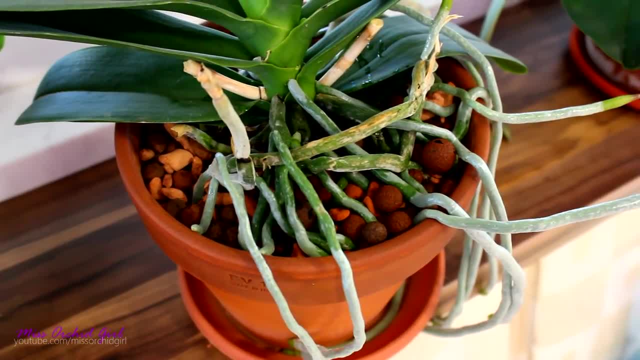 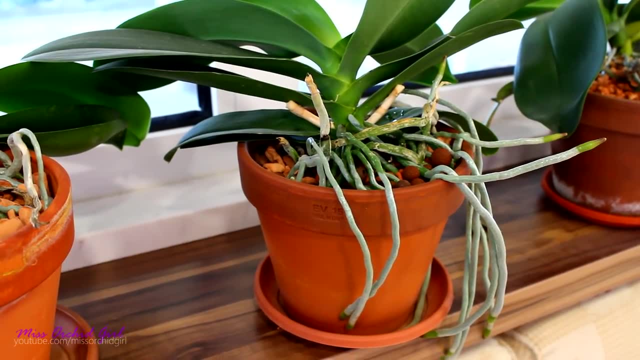 great. So as long as you have roots growing and swirling inside the pot and also roots growing outside the pot, you cannot say it is a pattern. And if the roots inside the medium are very healthy, you cannot say that the medium is inappropriate. Also, I can understand. 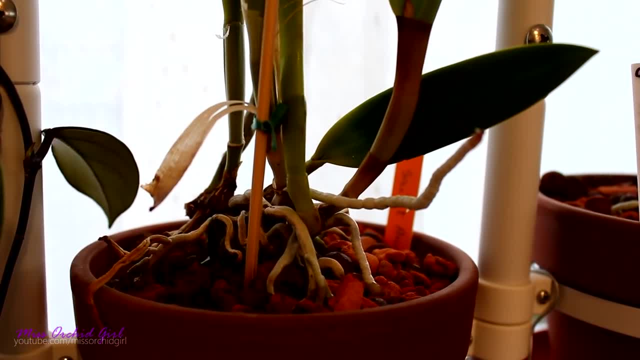 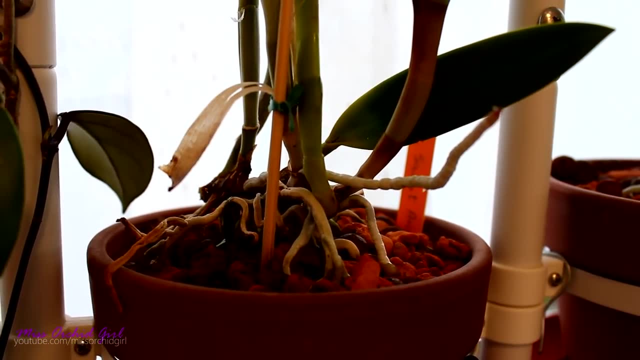 that in high light conditions and high temperatures roots might start to grow away from the light, But that's simply because they might overheat in the light. But you cannot really say that. it's a definite rule and all the roots on all of your orchids will grow away from the 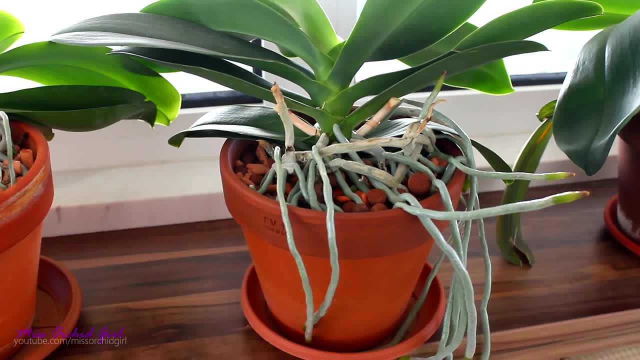 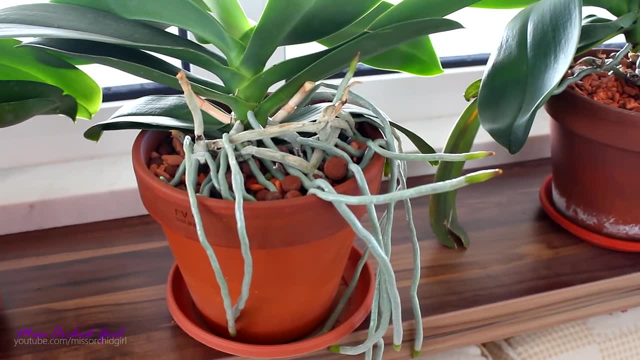 light. No, it is rather a random pattern. Now you might be tempted to ask: but Dani, why would an orchid root avoid a more moisture part of the tree? Isn't it in the orchid's interest to stay hydrated? Well, here's where. 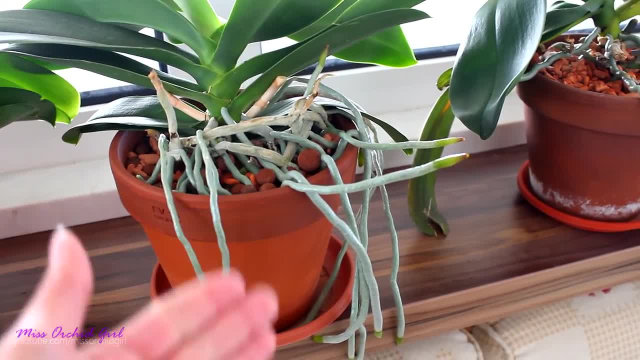 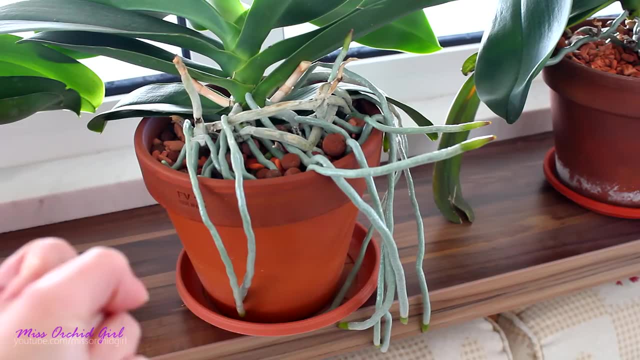 a nice little feature of orchid roots comes into play: They can adapt to various types of environments. This means that you will have roots which are more adapted to higher humidity conditions and some roots that are more suitable for higher humidity conditions. This means that you will have roots which are more adapted to higher humidity conditions. 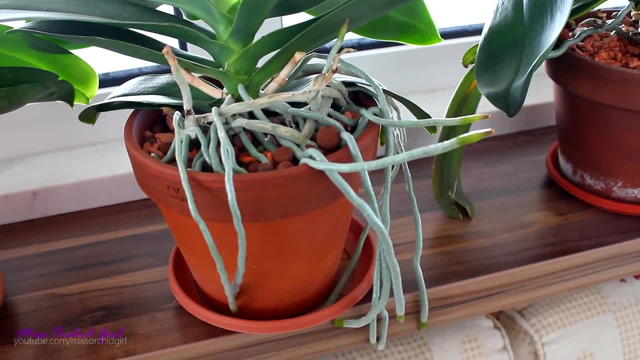 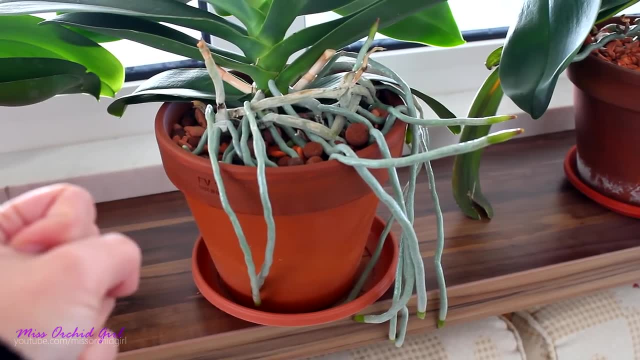 and some roots which are adapted perfectly to some lower humidity environments. And in the case of our orchids, you might already notice that the roots inside the pot do very well in high moisture, while the aerial roots do extremely well- just as well actually. 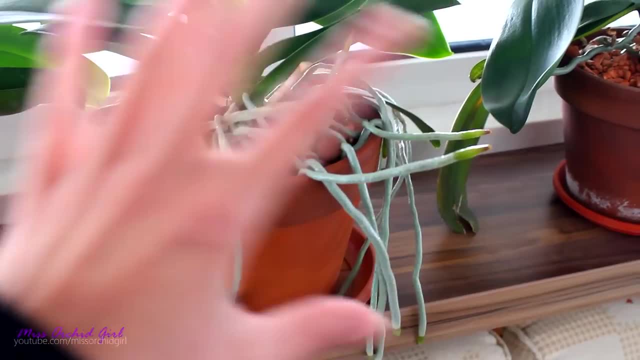 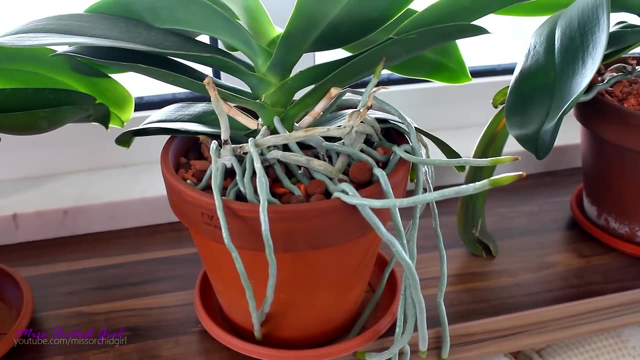 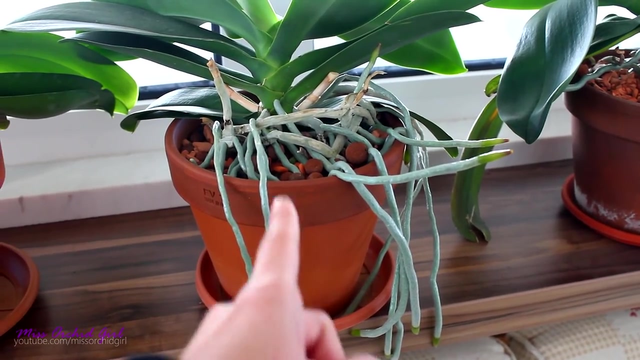 as the potted roots, And I am not referring here to extremes, not referring to environments with super dry air. So orchid roots are adaptable to various environments and various conditions in those environments. Now this feature has a little drawback in the case of our potted orchids. If you are going to try to pot an aerial root in many 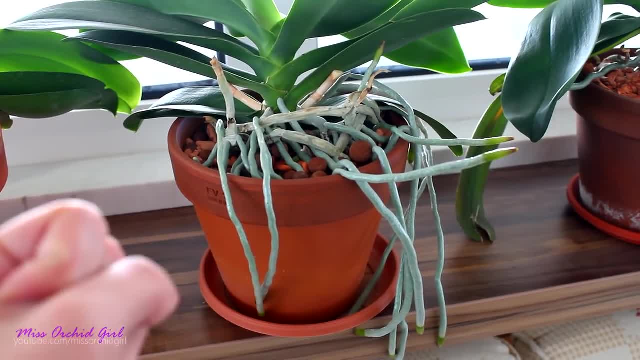 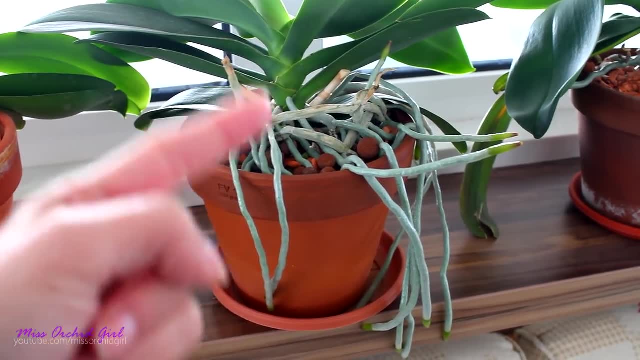 cases it will not do so great, because it is not adapted to that high amount of moisture and that low amount of air. Likewise, if you try to pull out from the pot a root adapted to life in a pot, it will probably dry out in air because it is not adapted to such 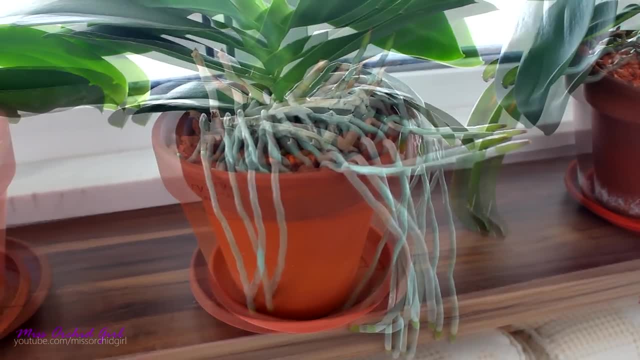 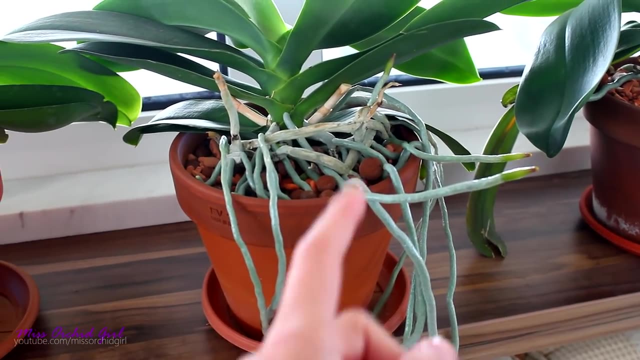 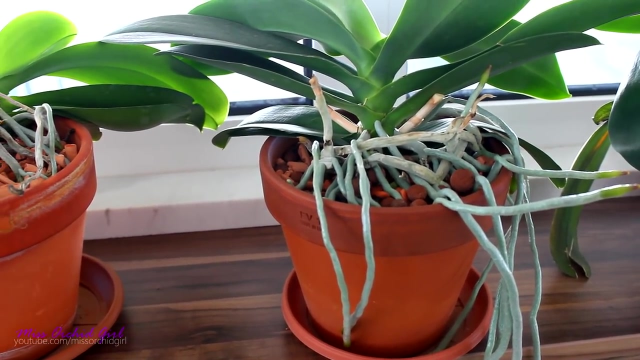 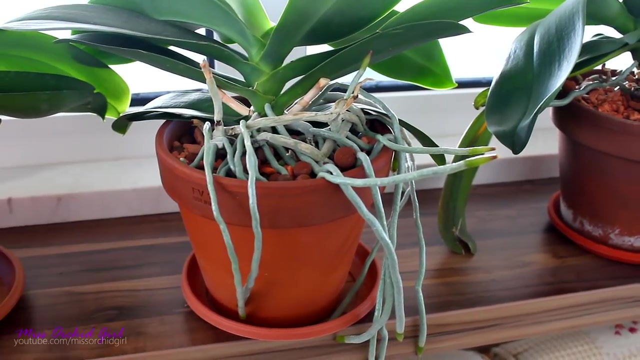 ventilation and air quantity and low humidity and so on. But this explains how roots can grow towards the moisture and in moist soil. So if you are going to try to pot an aerial root, you will need to use the roots that grow very well in the air in a lower moisture. 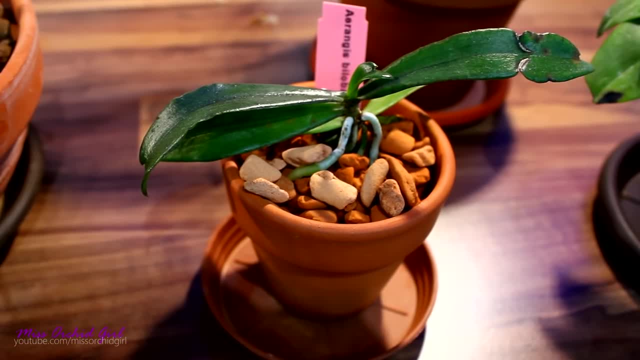 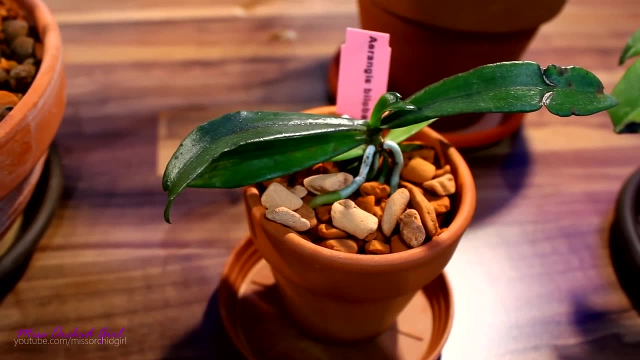 environment. So why all of these theories about what orchids want, where they grow and so on? Well, simply because we are human. We don't like randomness, because we cannot control it. We need to find uniformity and sense. 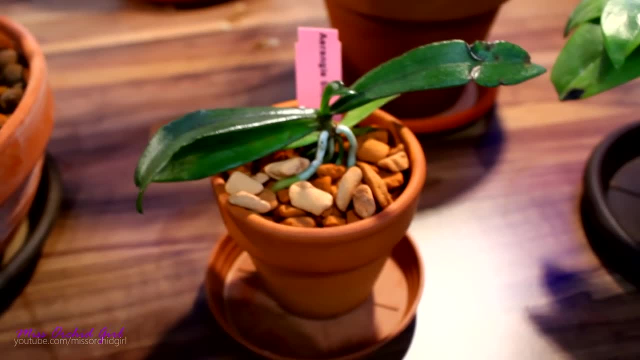 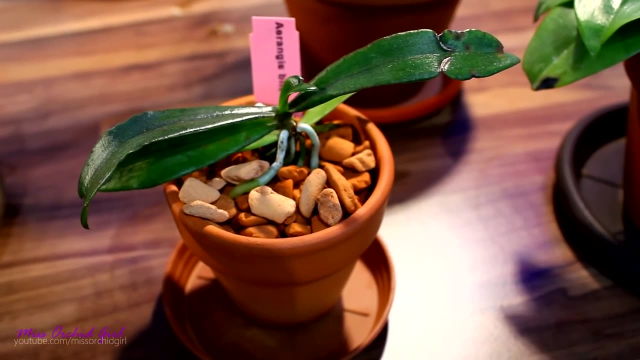 And giving a strict rule, such as roots tend to grow towards the moisture or towards the light and so on, makes things easier to understand and easier to control. But the truth of the matter is randomness has its own logic. The more random the growth pattern of roots is. 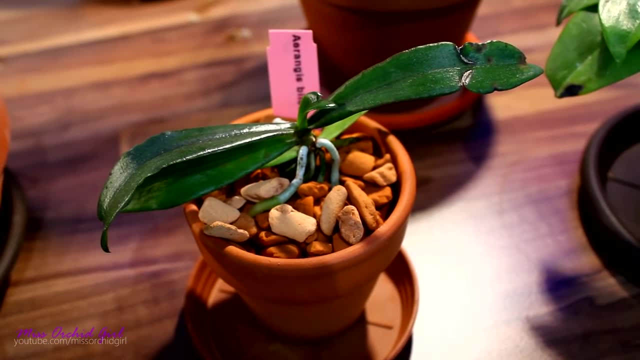 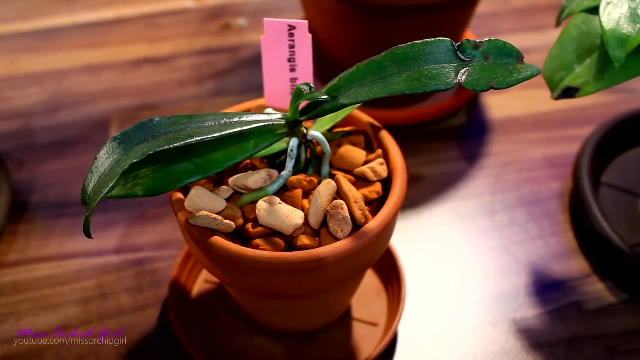 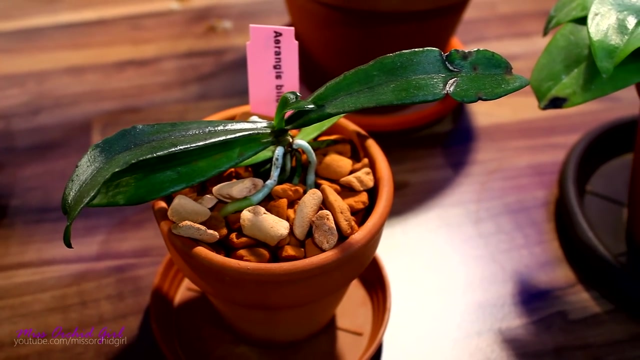 the better the orchid will get established, And for her this makes perfect, perfect sense. As I was saying, staying on that tree and in that location is a condition of survival. If an orchid root would follow these strict rules, it will be the death of her. So randomness for an orchid makes a lot more. 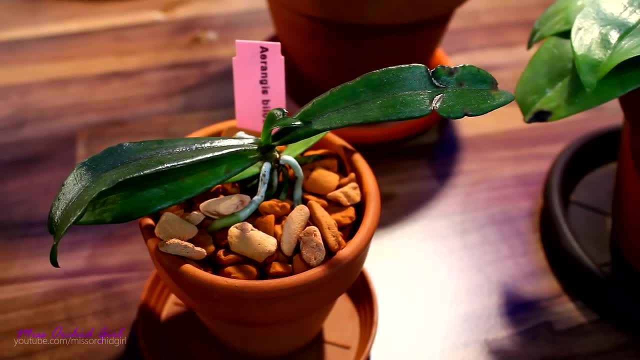 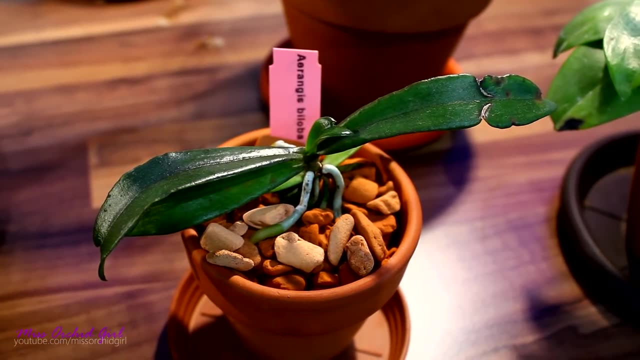 sense than for us. So I guess this is why we try to find reasons why stuff do this and do that- And I am guilty of that as well. I do like to find the reasons and the logic behind things. Sometimes those reasons are just a little bit more hard to. 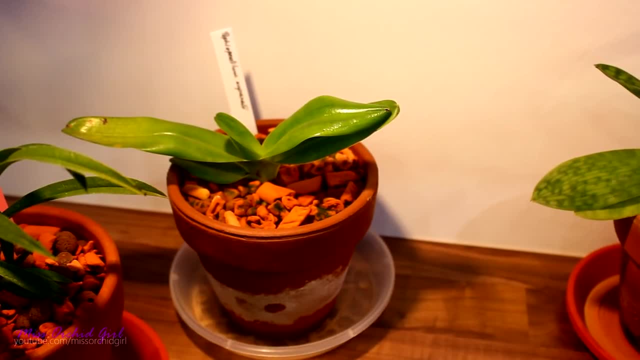 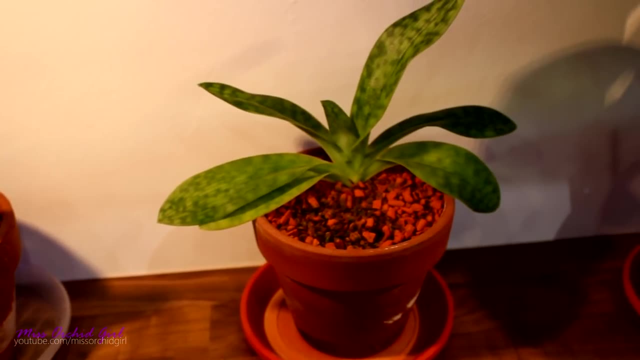 understand Doesn't mean they are not real. Now, in the case of terrestrial or semi-terrestrial orchids, you will not observe such behaviors, And the reason why is very simple: The roots of a terrestrial orchid simply do not like excessive amounts of air, So they grow away from the air. But 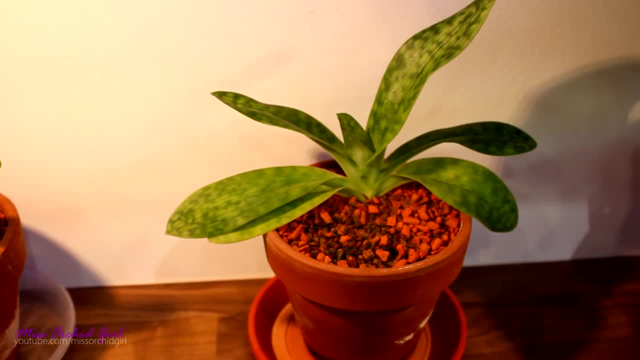 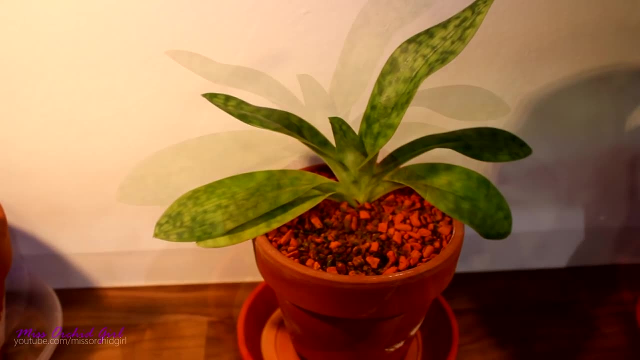 for the main part, you will never see aerial roots on terrestrial orchids, In any case not like with epiphytic orchids, Because they simply do not survive in that high amount of air. So with terrestrial orchids we can discuss. 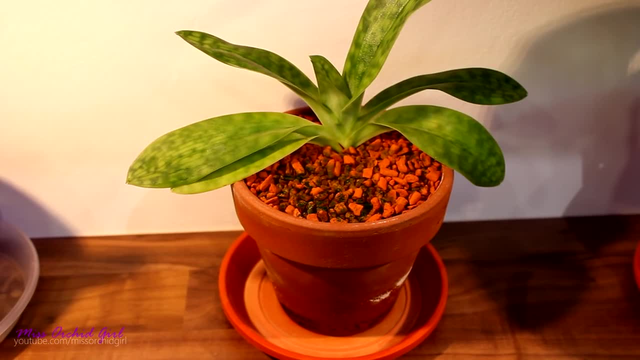 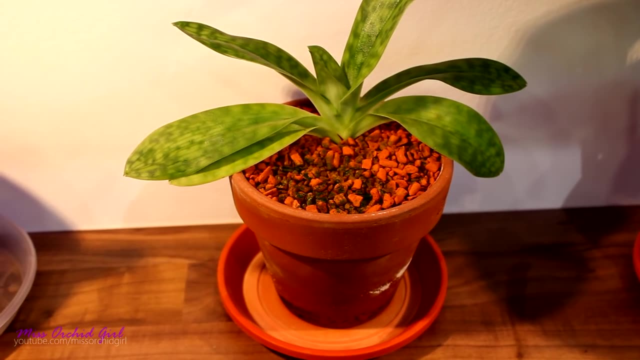 about a pattern of growth. They will tend to grow away from the light, meaning inside the soil. They will tend to grow where gravity pulls more, because that's usually where soil is, And they will also tend to grow where there is a little bit more moisture, not as 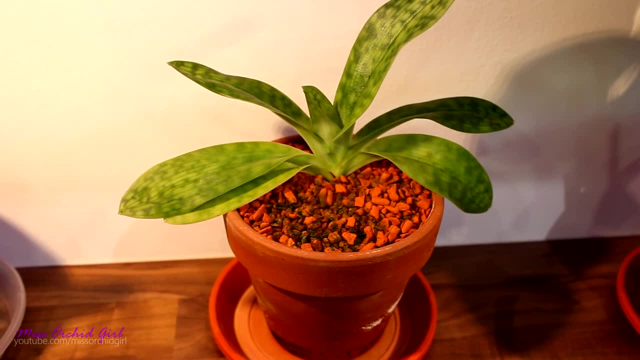 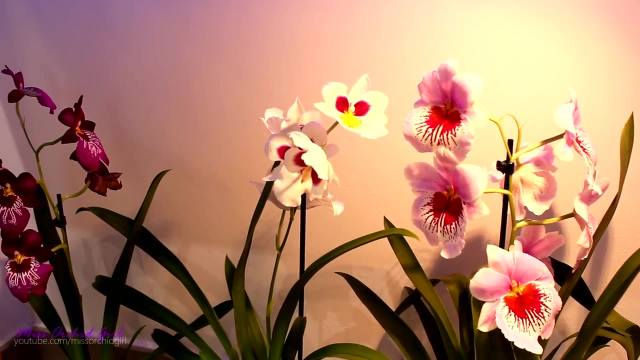 much air movement, And this pattern and behavior is similar to any other type of terrestrial plant, be it orchid or something else. Okay, guys, this is the video about roots. It's getting night here, so I think it's time to end. If I forgot to mention something, just feel free to leave me a comment down. 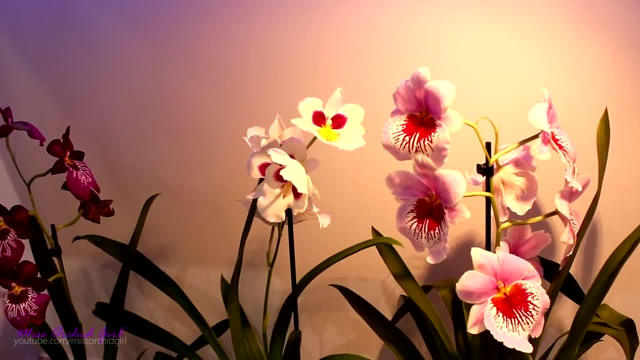 below. If you have questions, I will gladly answer and clarify things. Let me know down below what you think about things. Do you think that what I just said makes any sense? So if you've enjoyed this video, please give it a thumbs up And if you have any questions, 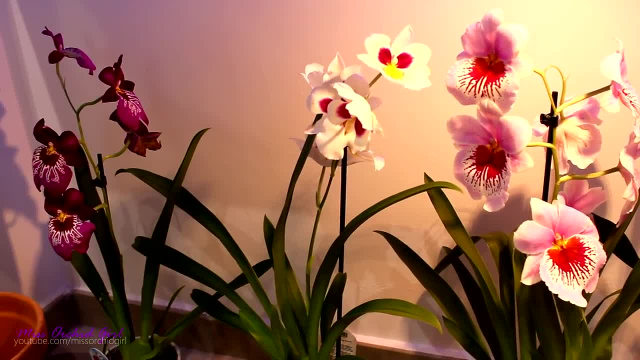 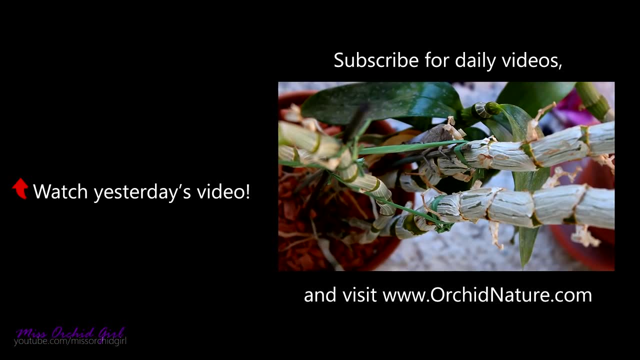 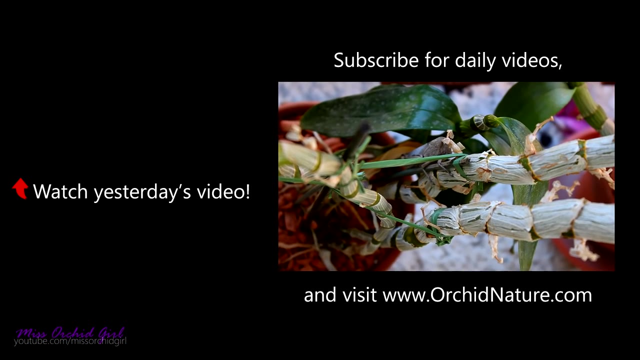 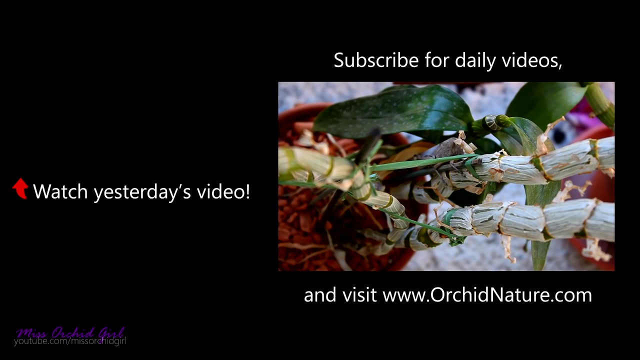 please give it a thumbs up. If you hate it, give it a thumbs down. Subscribe to my channel for daily orchid videos and I'll see you guys next time. Bye.